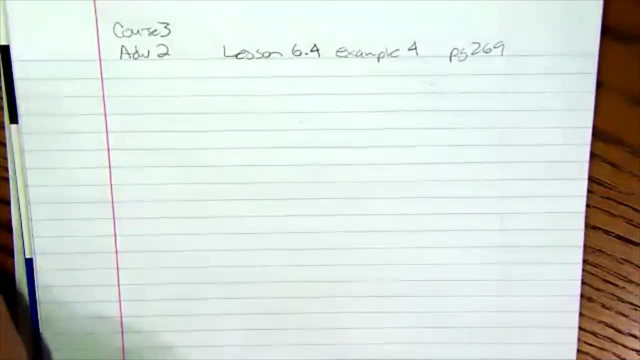 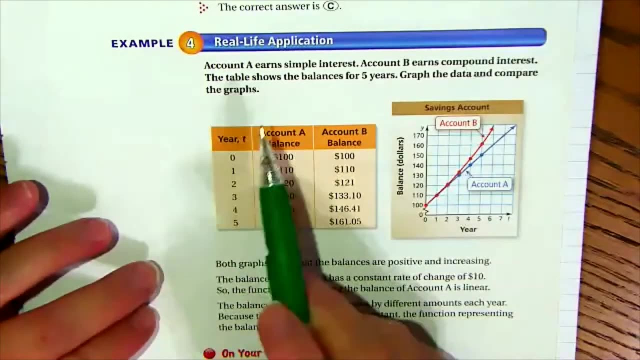 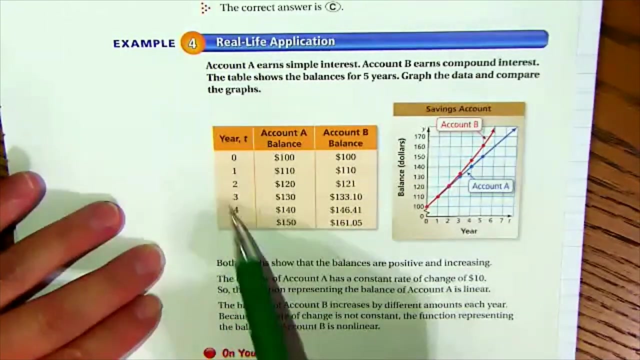 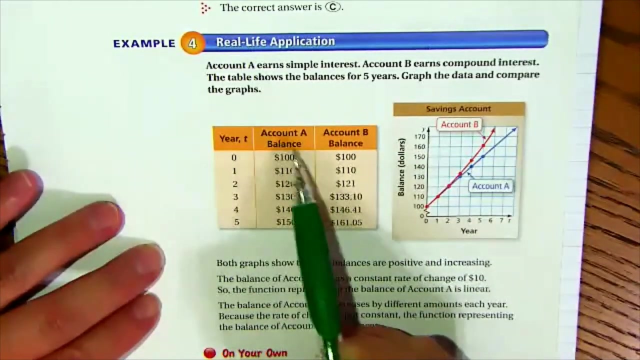 Today we're going to apply that to real-life situations. So let's take a look at this real-life situation. Account A earns simple interest. Account B earns compound interest. The table shows the balances for five years. Graph the data and compare the graphs. So account A is simple interest, Account B is compound. 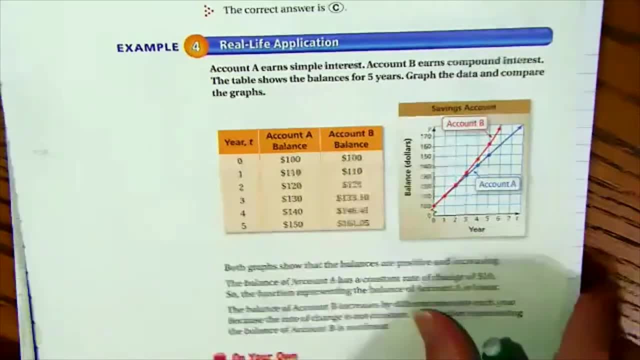 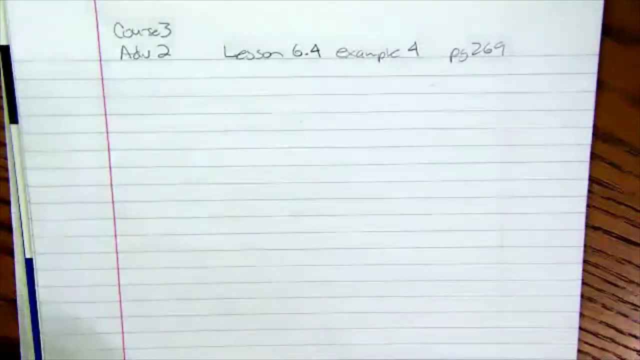 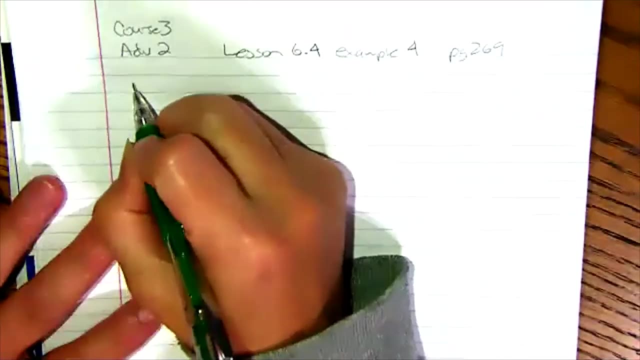 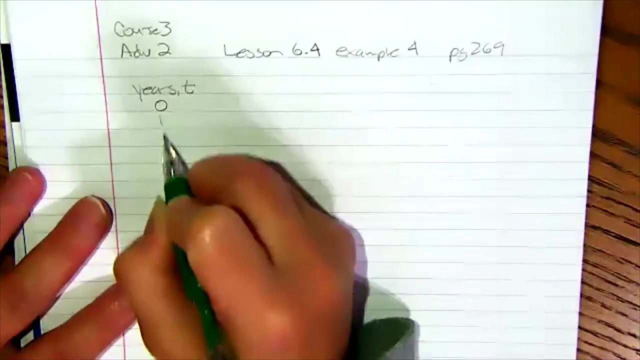 interest And account B is compound interest And account B is compound interest And account B is years are years. Okay, So let's go ahead and copy that down. So we have years which is represented by T Time zero, one, two, three, four, five. 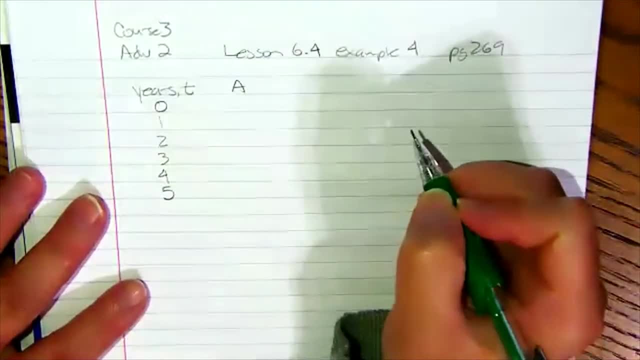 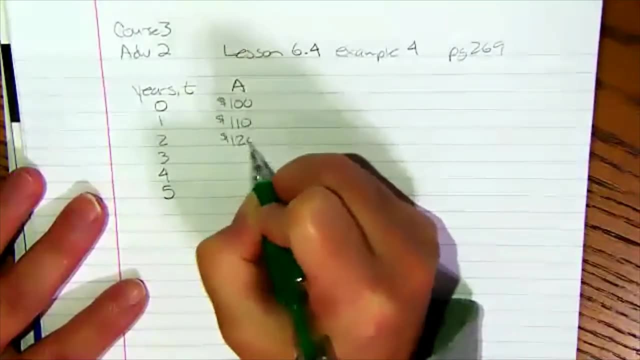 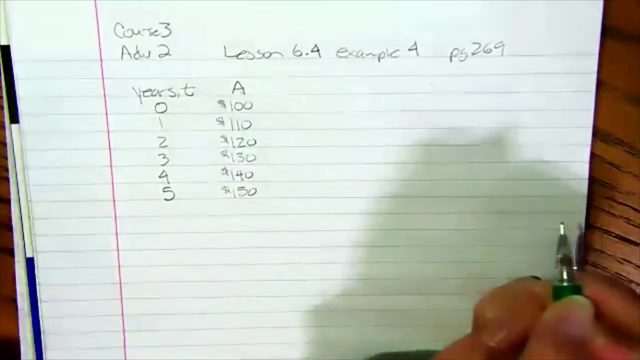 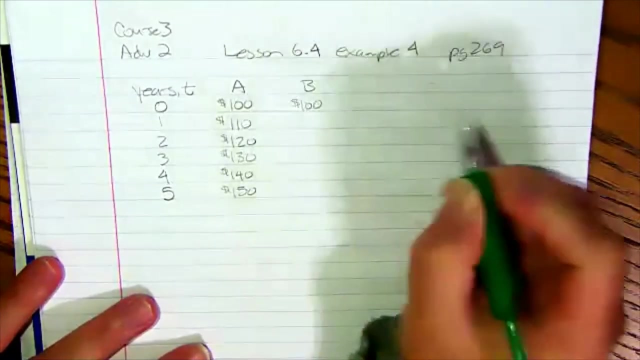 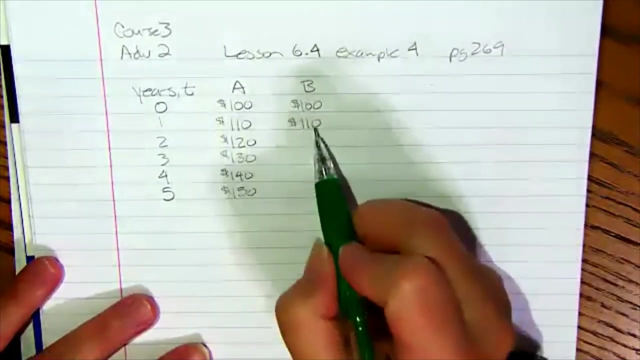 We have account A, which is simple interest, so we start with $100 and then every year we gain $10.. Then we have account B, which is compounded interest, which means the next year's interest is based on the year before. So the interest here is based on this. 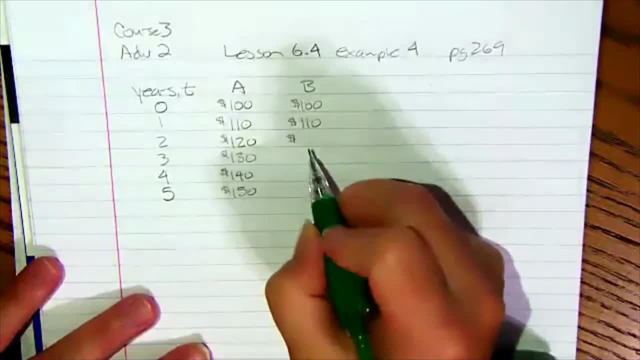 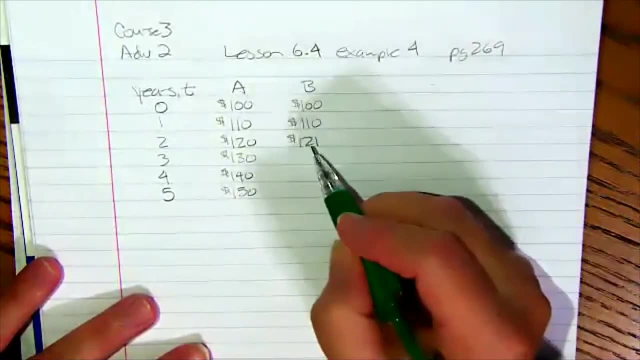 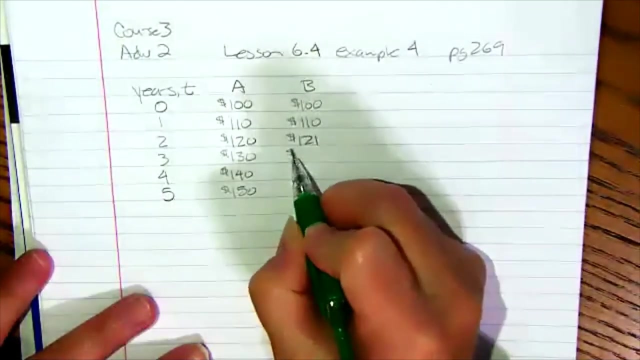 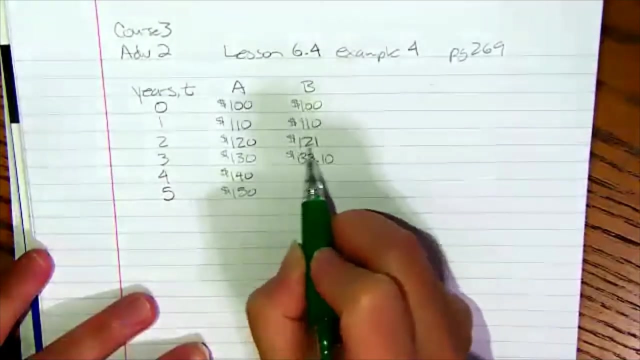 hundred dollars. but now the interest here is based on the hundred ten dollars. We're earning interest on that $10 interest as well. The interest here, interest here is based on this 121.. So we're earning interest on that initial $100, but on 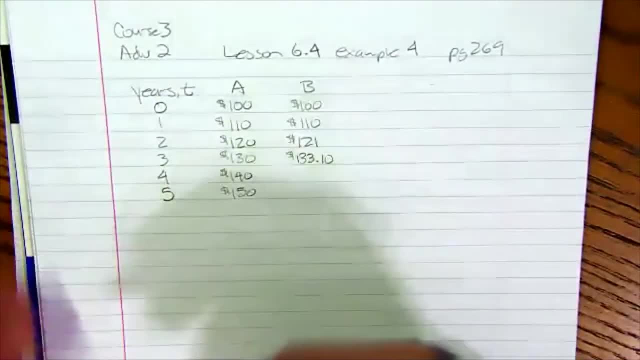 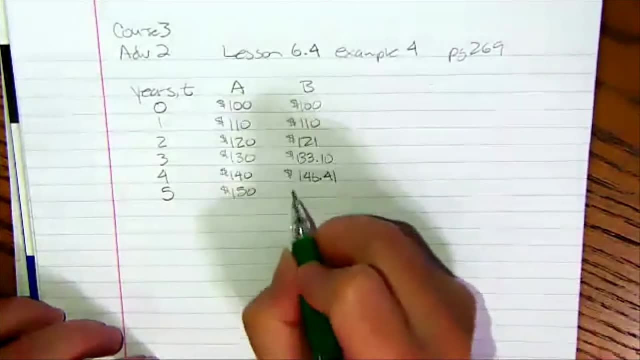 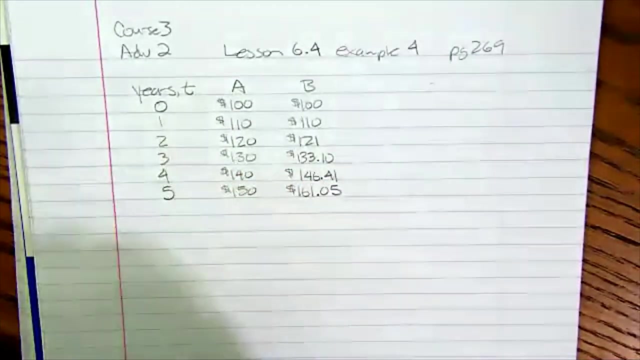 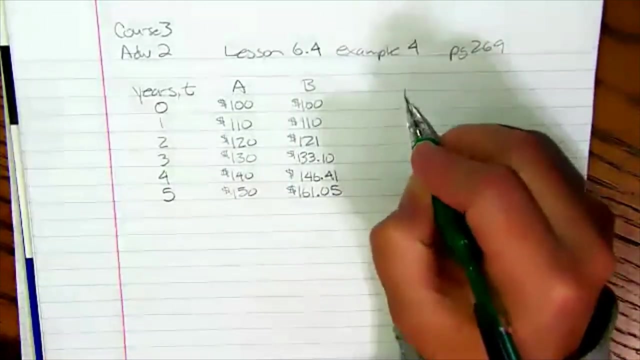 this $21 as well, So the interest is compounding, Okay. so here's the table that the book has given us Years. account A is simple interest. account B is compound interest, and they wanted us to graph this and compare the graphs. Okay, sounds easy enough. Okay, since I don't have any negatives. 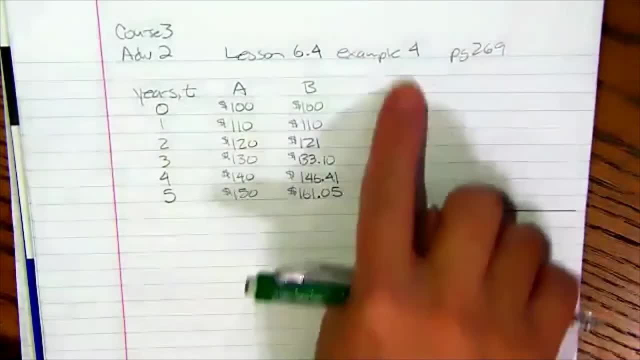 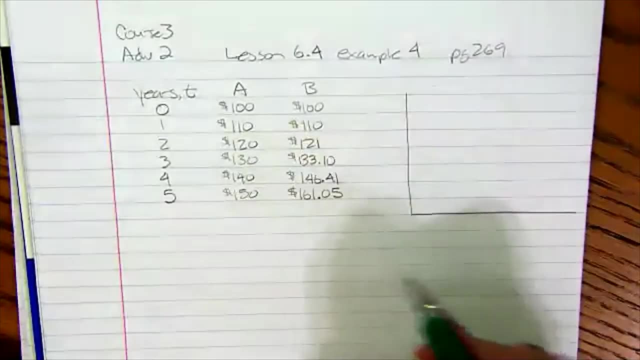 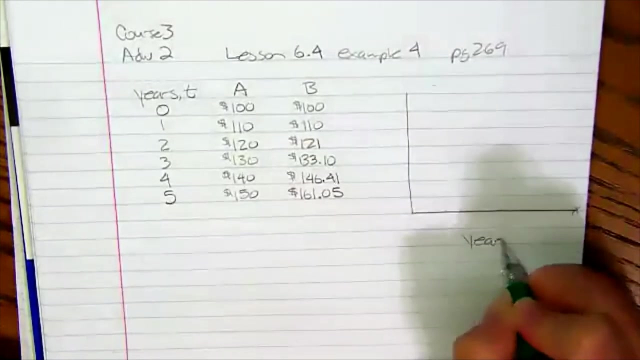 I'm not going to be working in any of the negative spaces, I only need the first quadrant. So my graph is only going to have the first quadrant because I don't have any negatives. So my x is going to be years Right here. this is my x, So I have one, two. 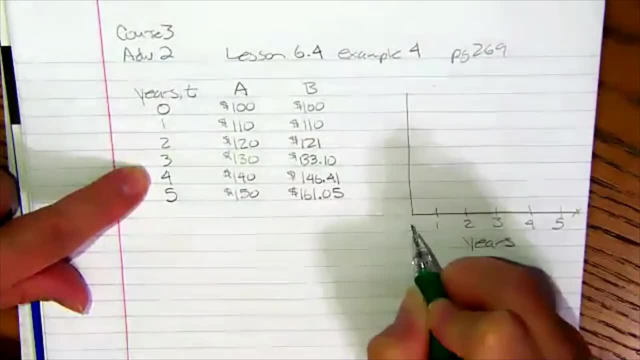 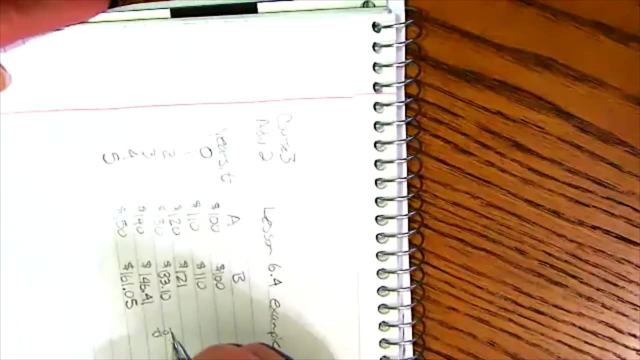 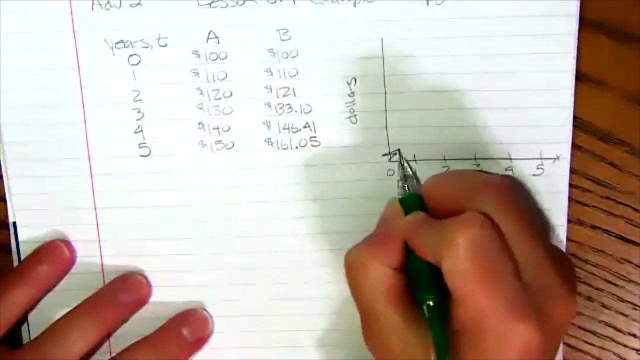 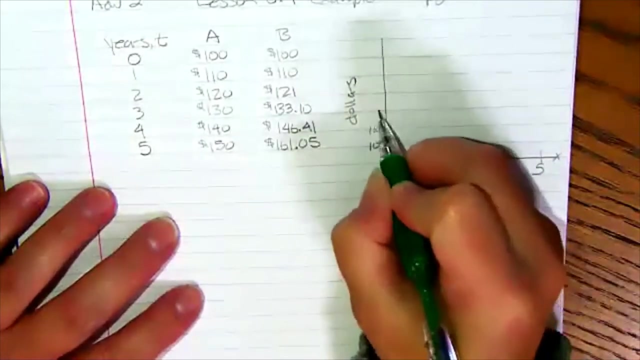 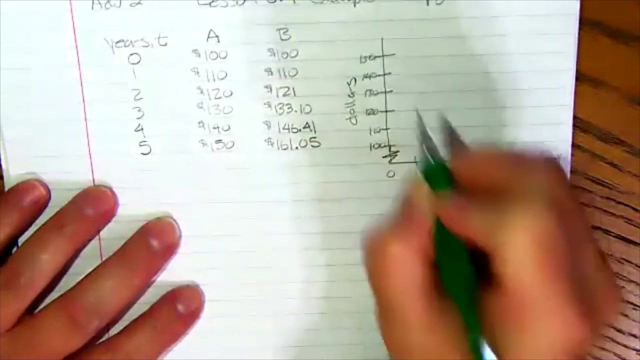 three, four, five. My y-axis is going to be dollars And And We're going to start with 100, 110, 120, 130, 140, 150, 160.. So we're going to graph these bad. 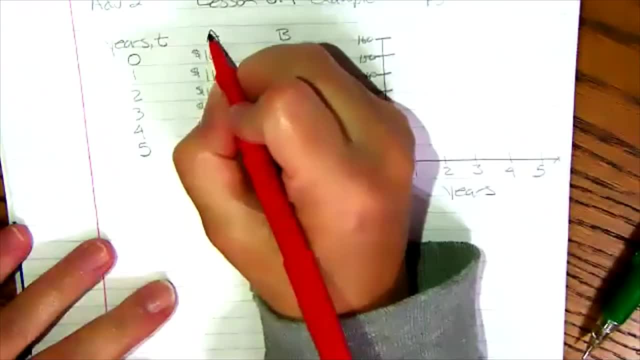 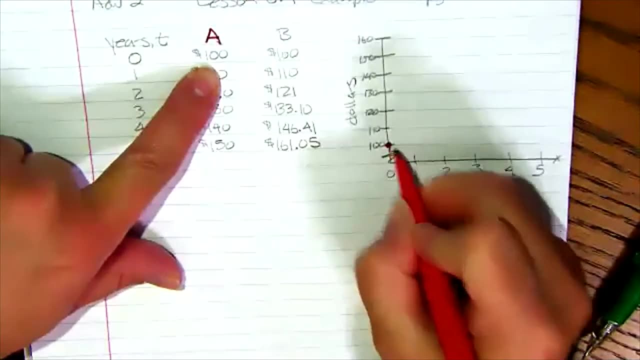 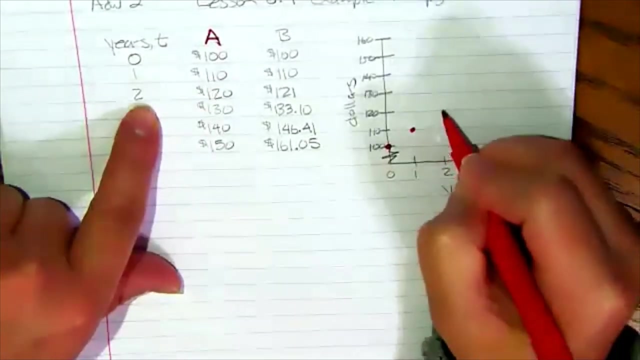 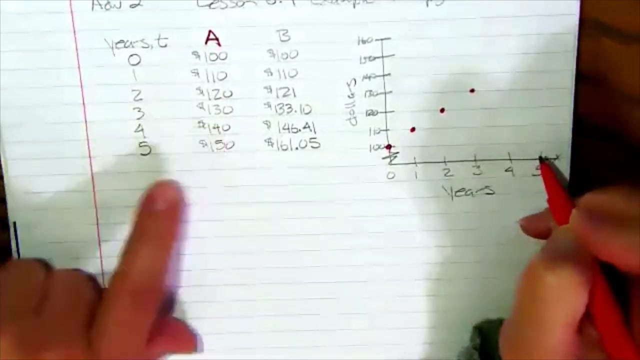 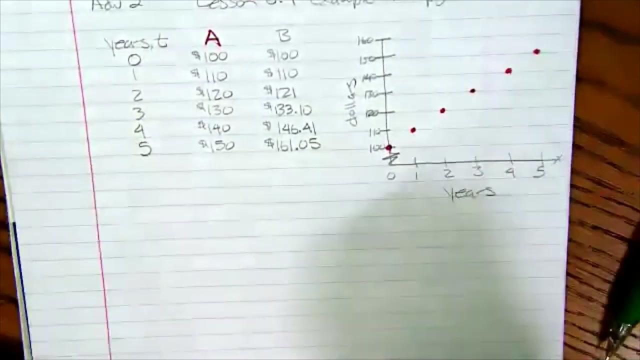 boys. So first let's graph account. A simple interest: Zero years $100.. One year $110.. Two years $120.. Three years $130.. Four years $140.. And five years $150.. 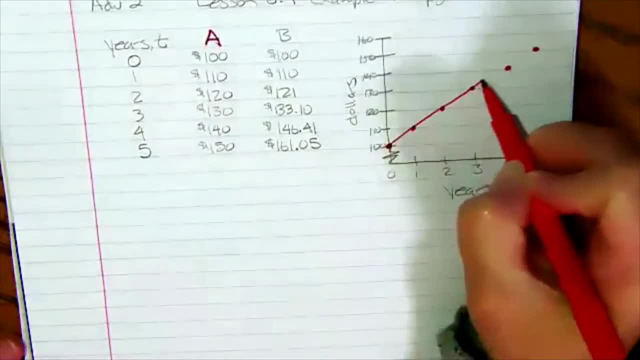 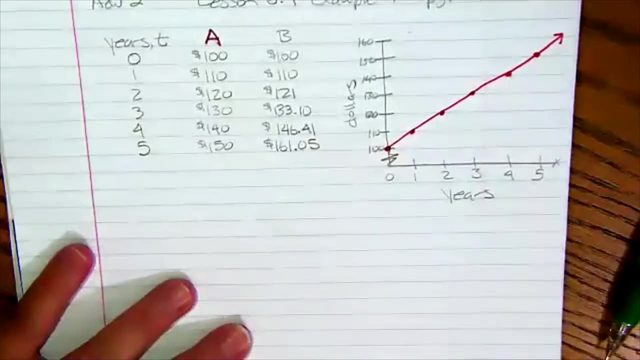 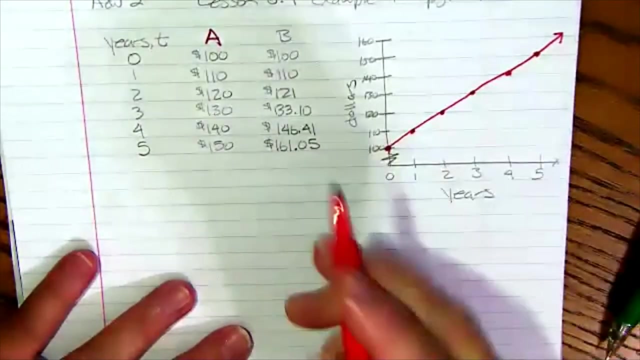 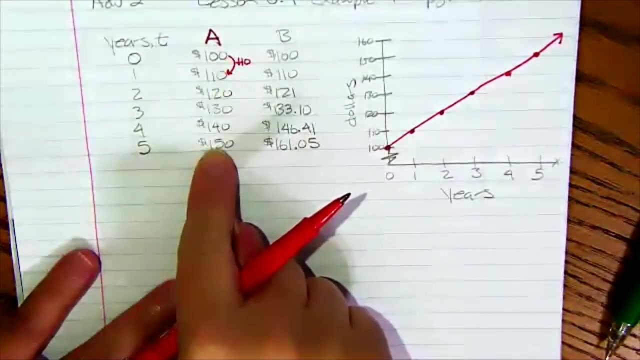 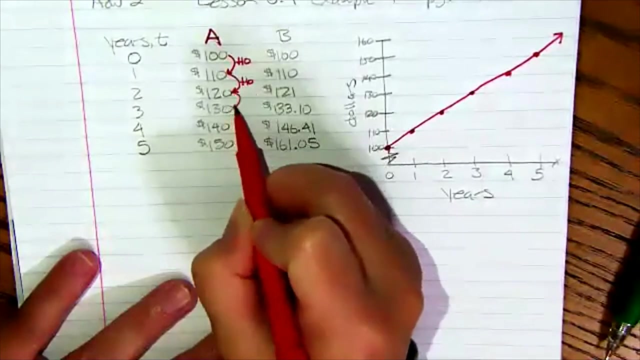 So when I look at this, that graph looks pretty, pretty straight to me. It looks pretty linear. But just to confirm that this is linear, that it is straight, I'm going to check my rate of change here. So, plus 10,, plus 10,, plus 10.. Ah, And it. 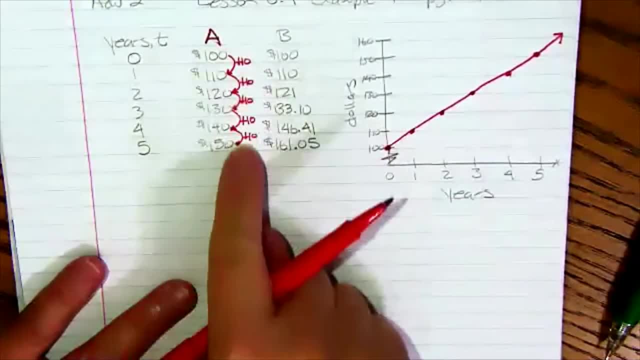 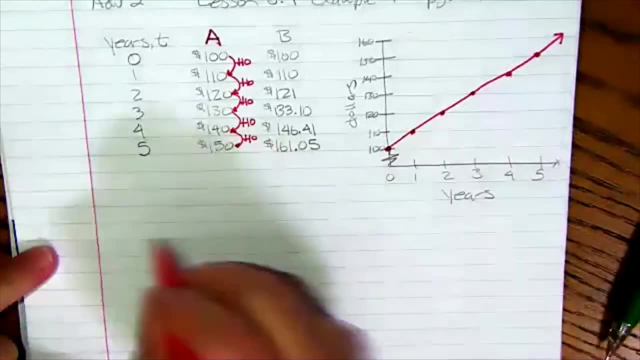 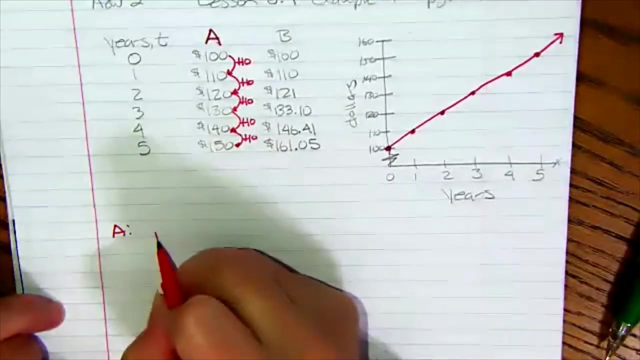 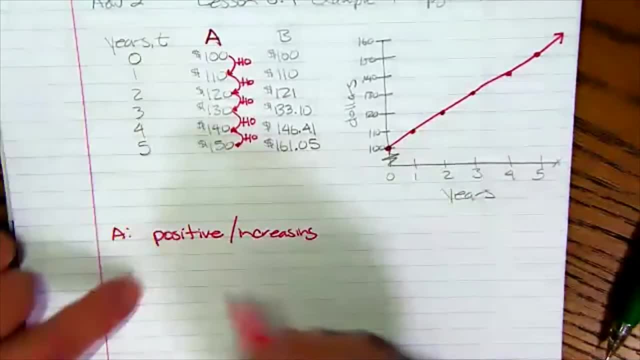 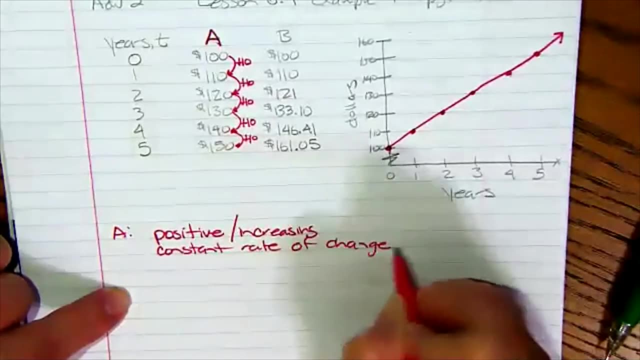 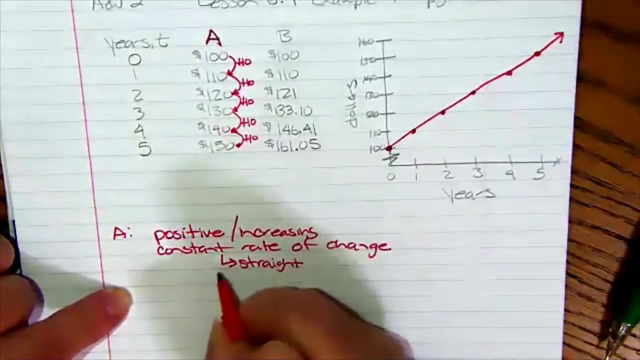 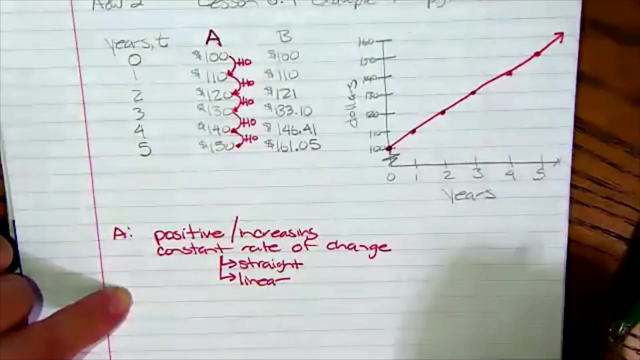 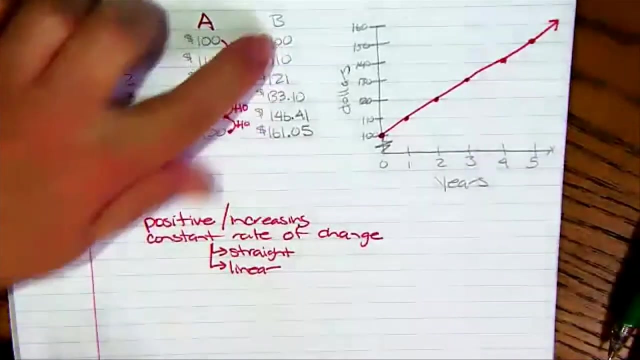 I can see that I have a constant rate of change, rate of change, And that means that my graph is straight, Which means this is a linear function. OK, Now. ok, Now, let's graph account B. that has compound interest. 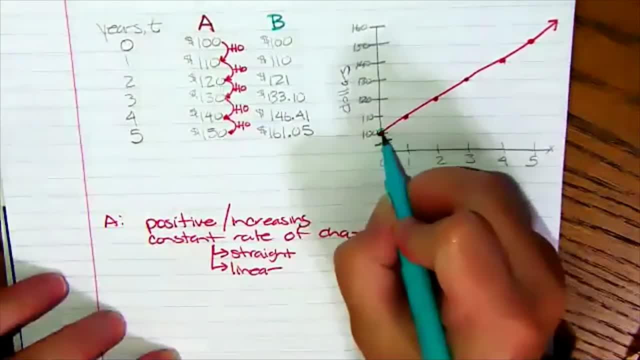 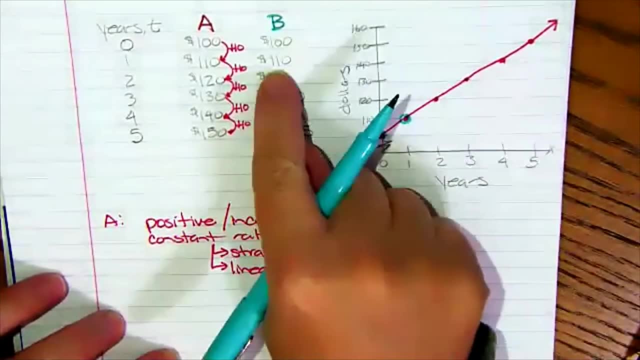 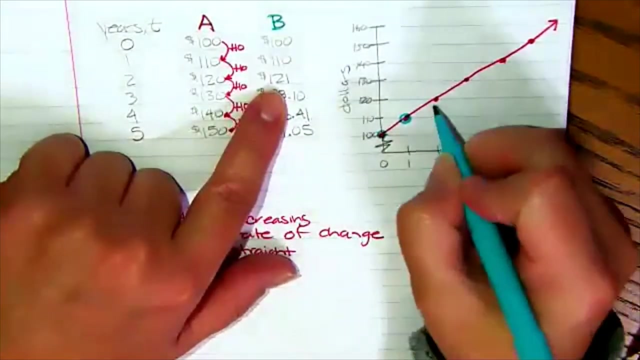 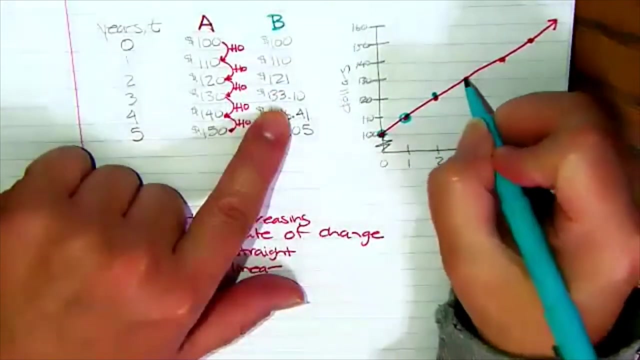 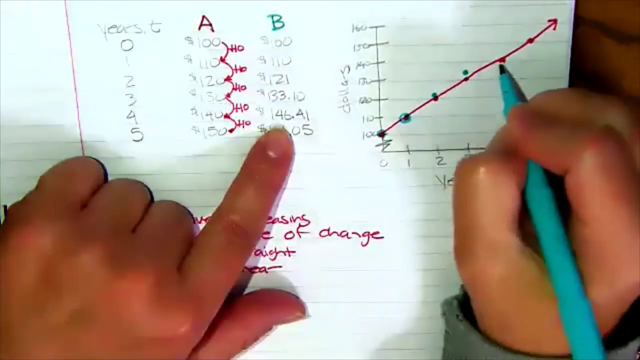 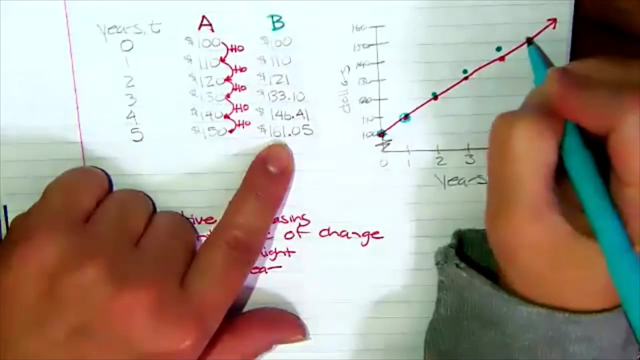 So we have zero and one. So at zero years we deposit $100.. After one year we have $110, just like account A. But now this is where we start differing. After two years we have $121.. After three years we've got $33.10.. After four years we have $146.. And after five years we have $161.. 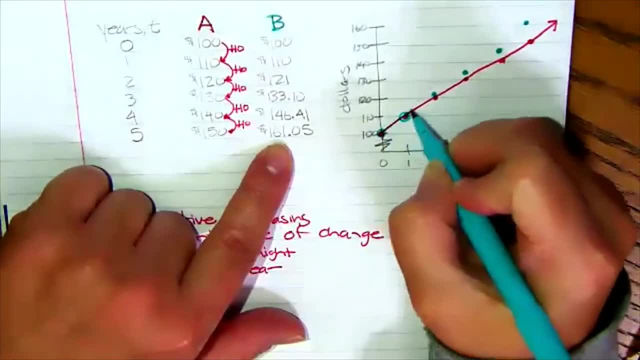 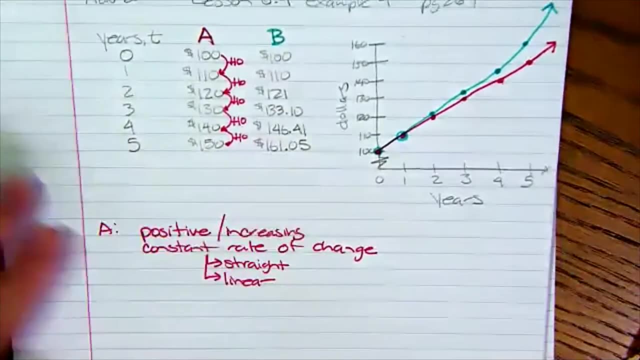 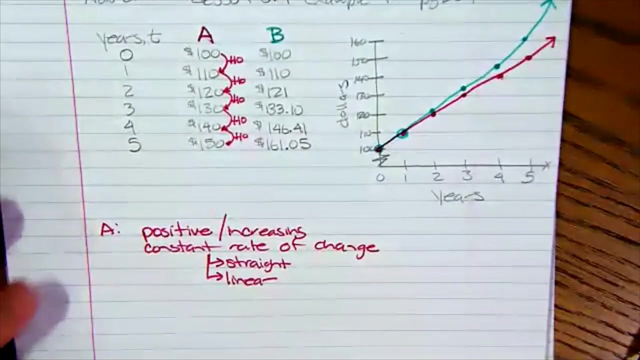 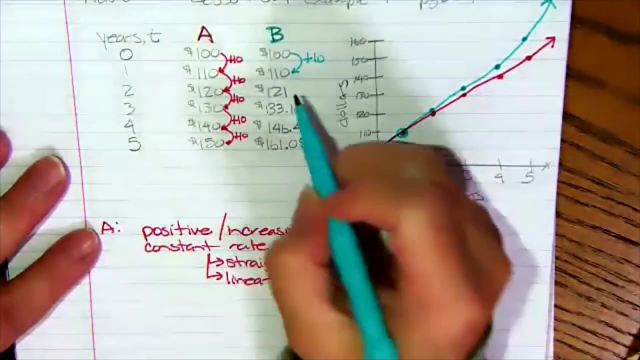 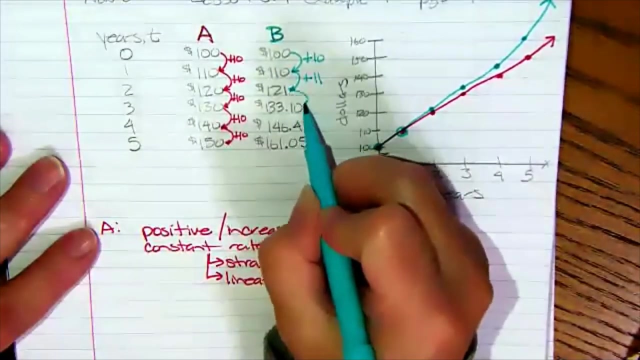 When I look at this, that line doesn't look very straight to me. It looks like it kind of curves. But just to be sure I'm going to check my rate of change: Plus 10.. Ah, plus 11.. Plus 11.. 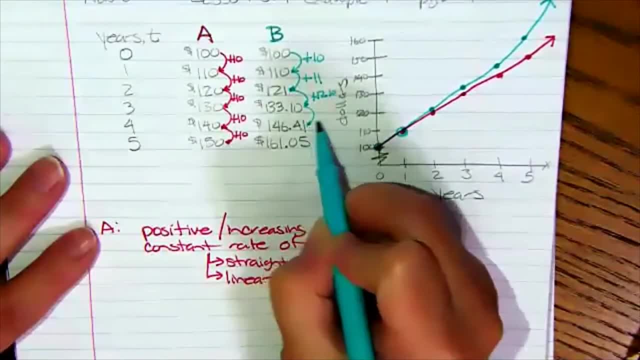 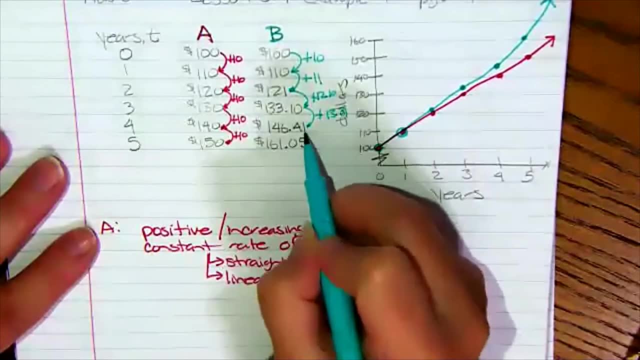 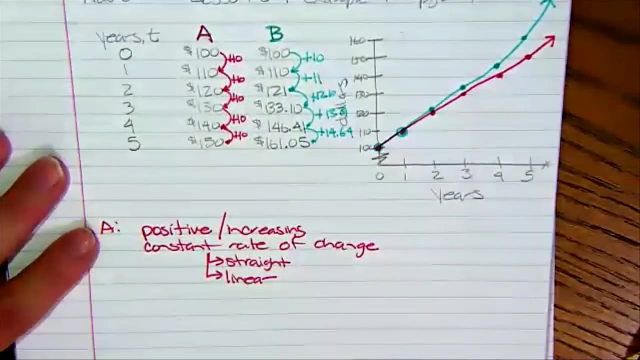 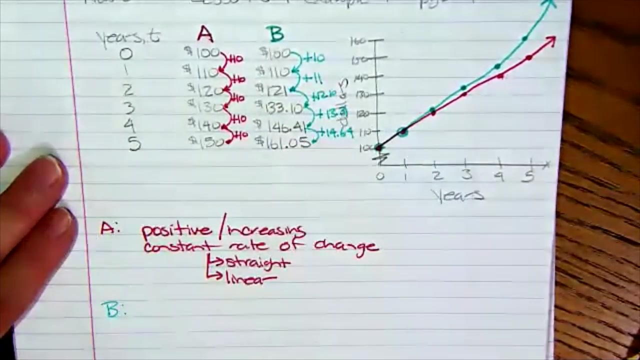 Plus $12.10.. Plus $13.31.. Plus $14.64.. This is not. there is a pattern here, but it is not a constant rate of change. It's not constant. So what's going on here with the 80%? 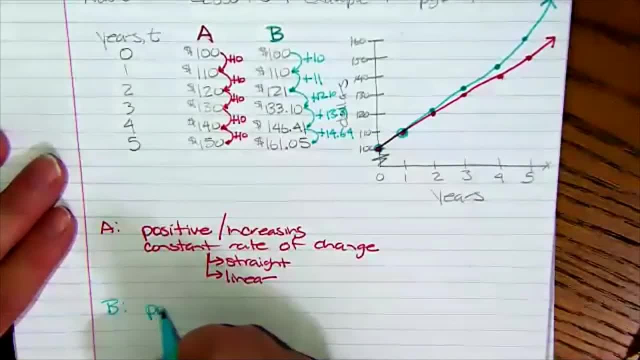 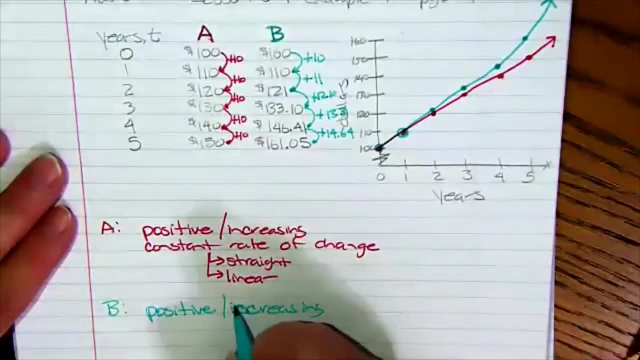 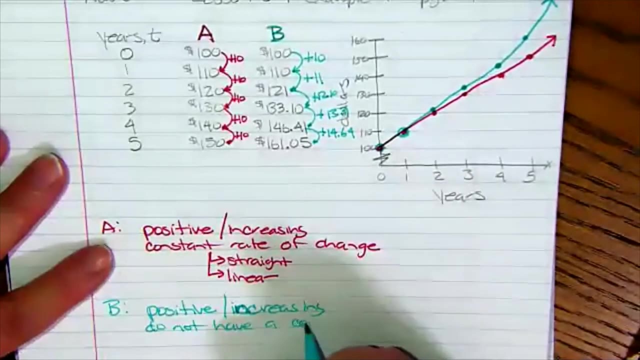 So I can see that my graph is positive. My graph is negative. The amount is still increasing. The increase of my salary Will begin next week, But I don't have the constant rate of change. But in blue I tell you I'm 400%. 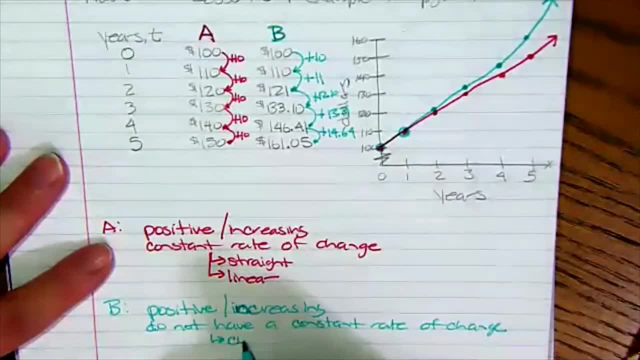 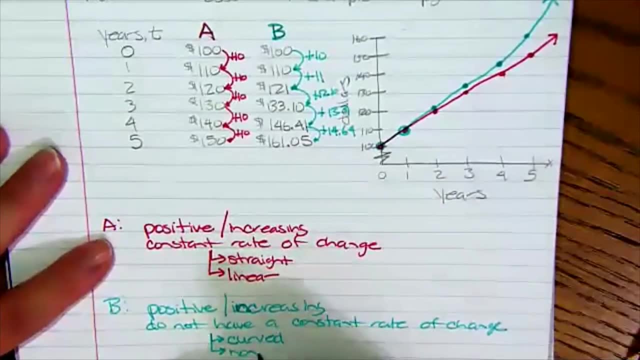 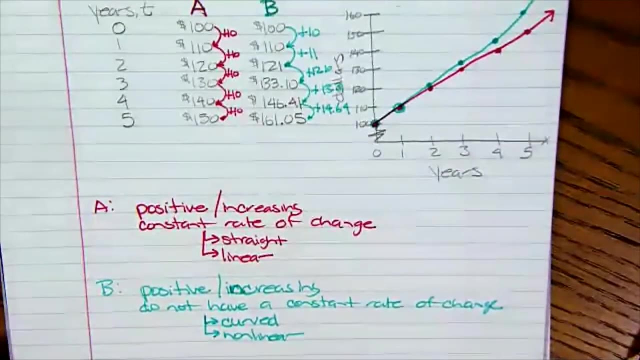 So I don't. It's positive. So if I look at my graph, I can see that it is curved, which means this is a non-linear function And this is real life. People are like: when are we going to use linear and non-linear functions? 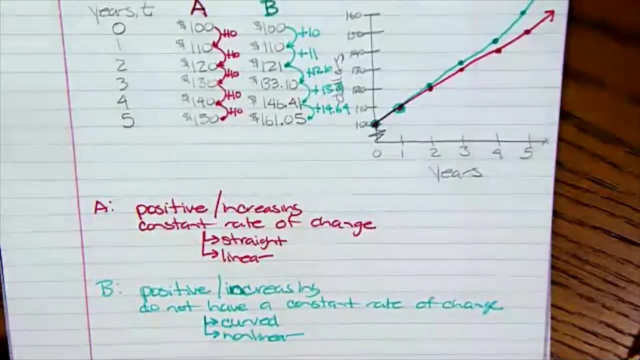 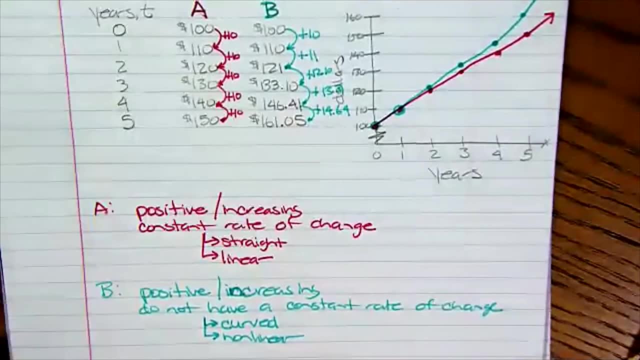 Well, banks use them every day to determine simple interest versus compound interest. How does this affect you? One of these days, I hope, you plan on retiring. get a job, get a career. You're making money, You're setting money aside so that one day you can retire. 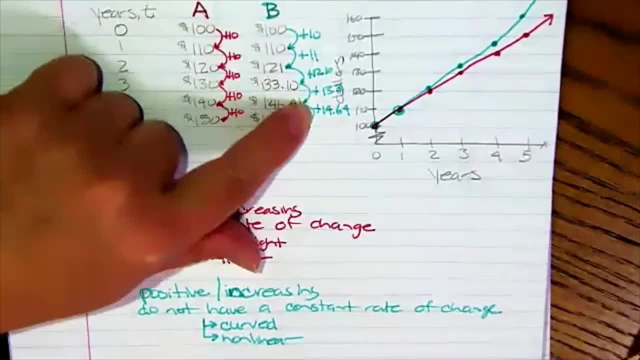 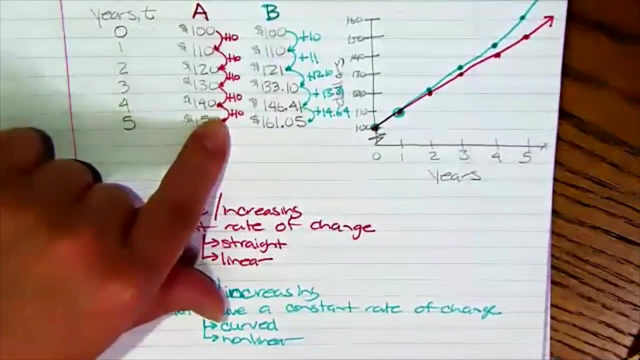 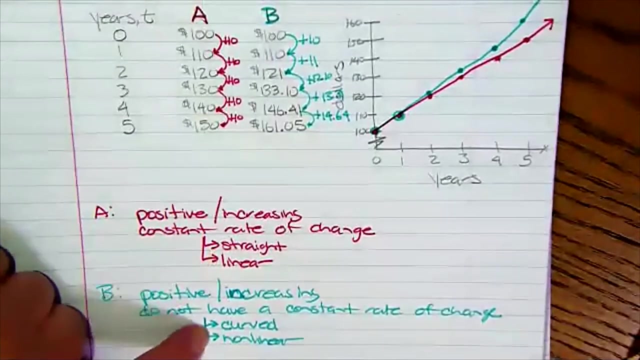 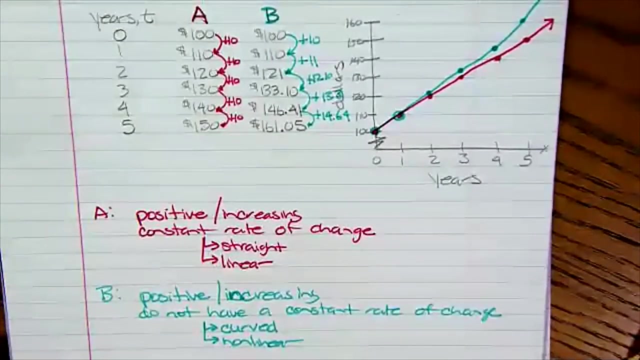 You want to be working with compound interest because you make more money quicker than you make money- And simple interest. So here is an example of a real life application of linear versus non-linear functions. Okay, The math is real, So let's do another one. 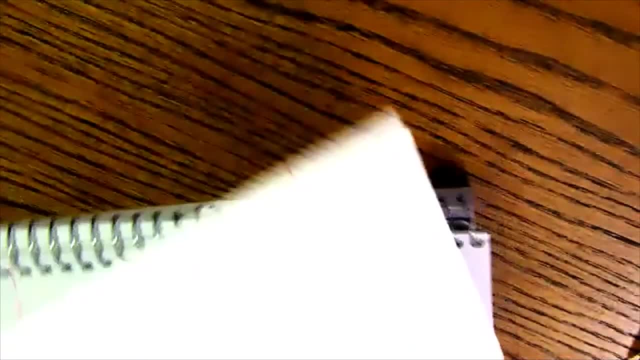 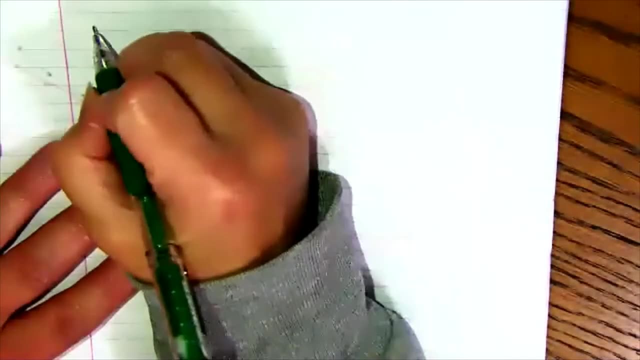 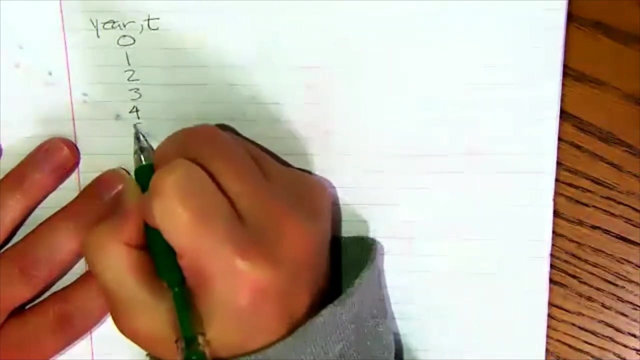 Let's do another example. Okay, The book is going to give us this, So the year again, which is time 0, 1,, 2,, 3,, 4, 5.. We have a count A, which is simple, interest. 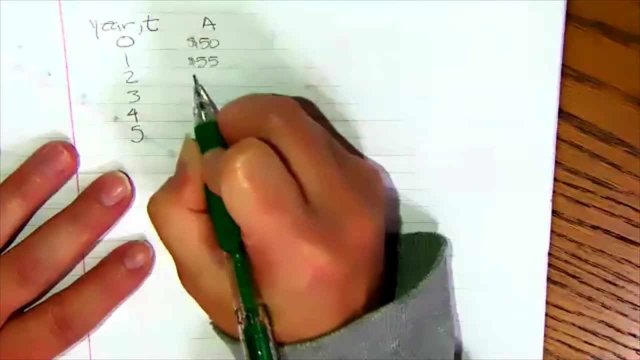 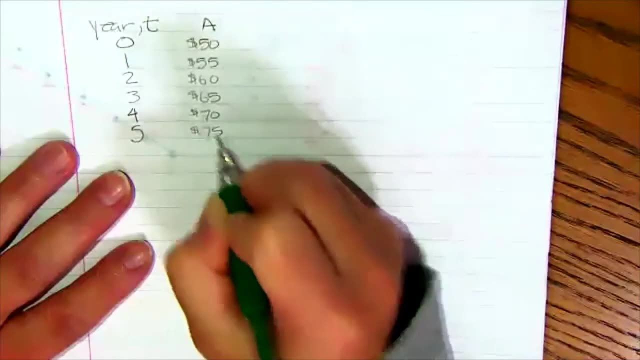 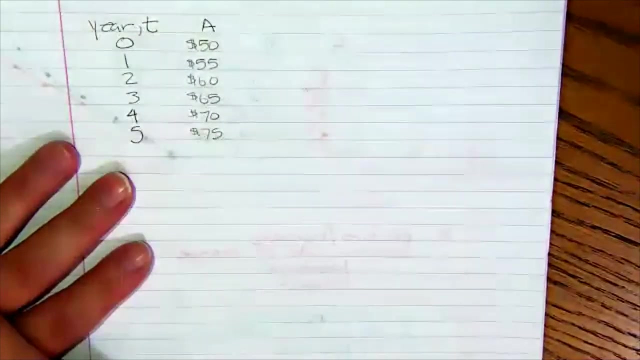 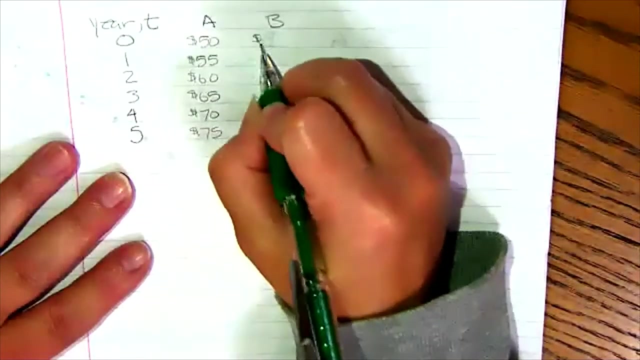 We start with $50.. And every year it grows by $5. Simple interest: Every year it grows by $5. It's guaranteed. Then we have a count B, which is compound interest. We start with $50, just like a count A. 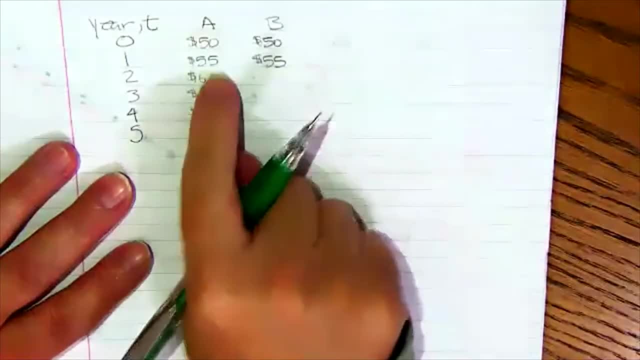 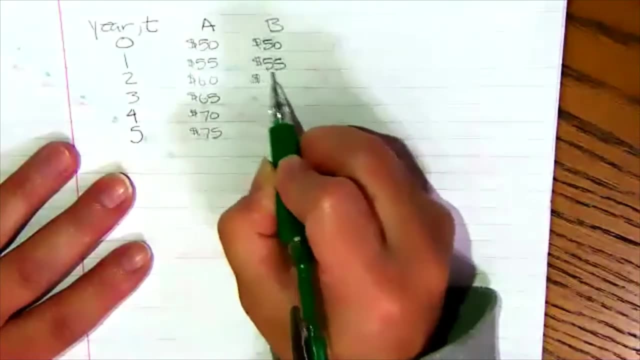 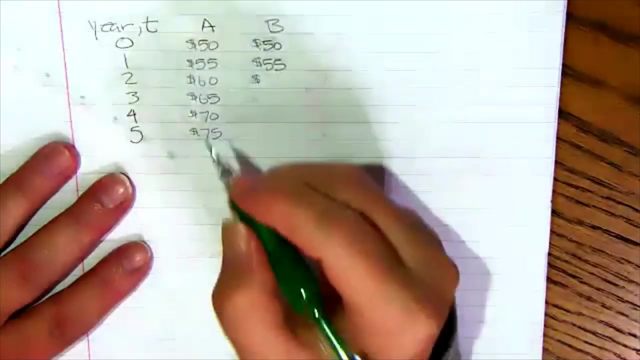 And after one year we have $55, just like a count A. But now we're earning interest on this whole amount, this $55. Not $50, but the $55. And you can see we've got $0.50 more. 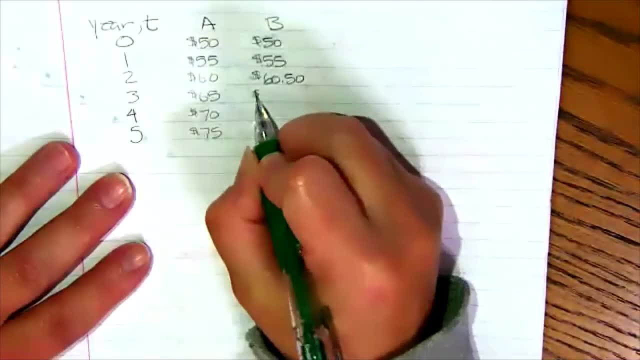 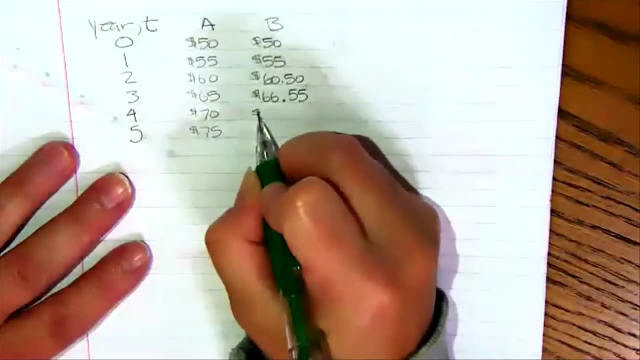 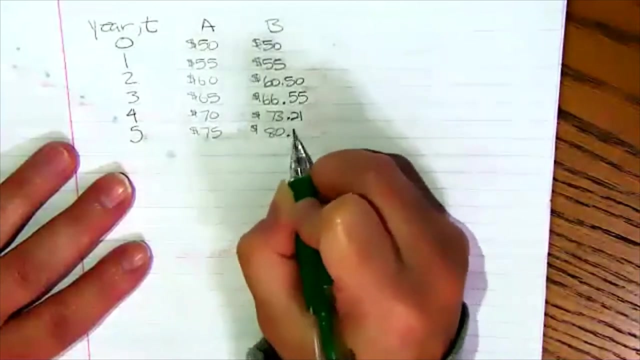 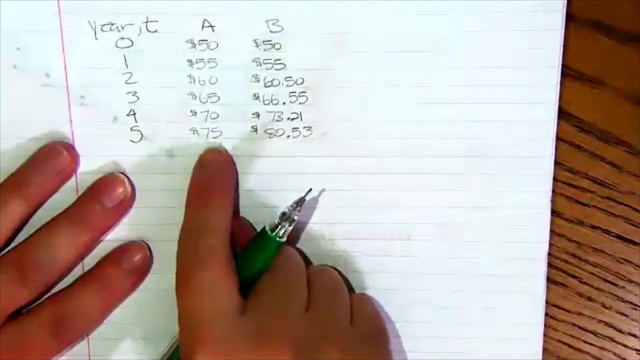 It doesn't look like that much. It's not that big of a deal, But over time it does become a big deal. So after five years we've got $5.. $5., $5.. More than $5,, more than a count A. 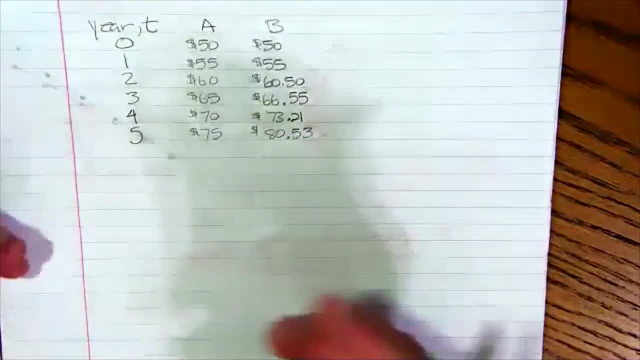 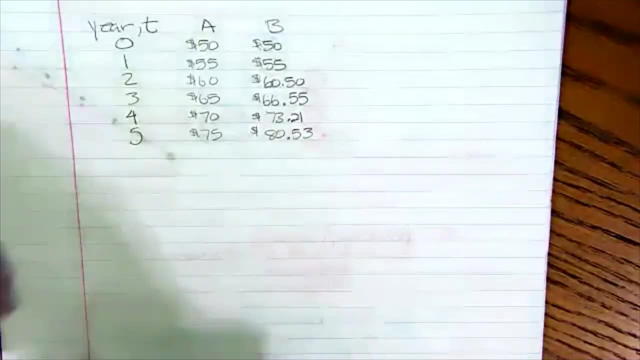 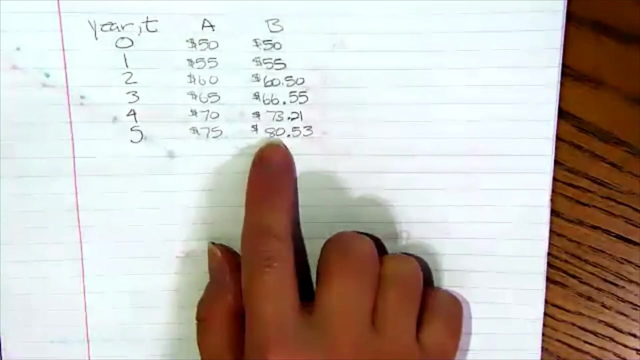 And this here is a small amount of money. You're thinking $5.. Yippee skippy. But what if this is your retirement and you're talking about tens of thousands or hundreds of thousands of dollars? This could be $500 more or $5,000 more or $50,000 more. 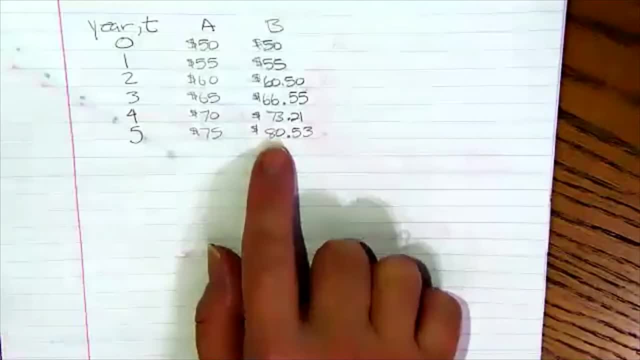 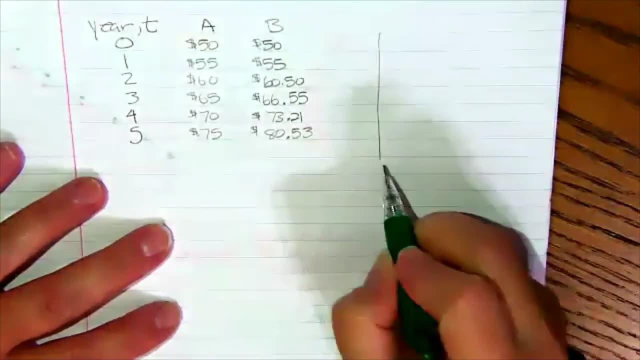 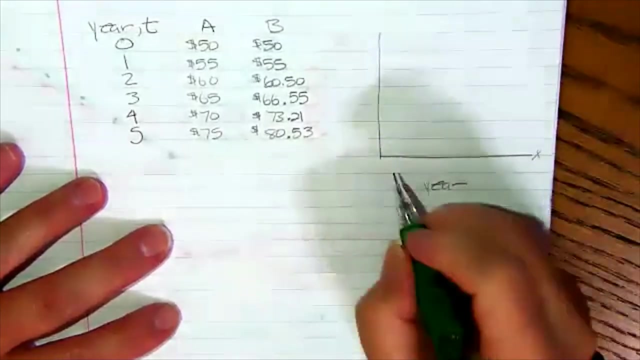 That's a lot of money. So compounded interest is kind of a big deal. So let's graph this and see what we've got. So here's my x-axis, This is the year, And I've got 1,, 2,, 3, 4, 5.. 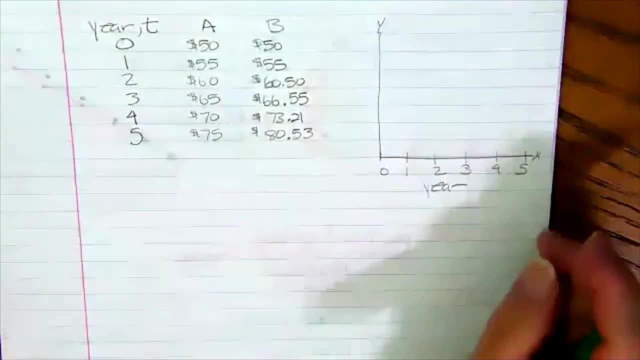 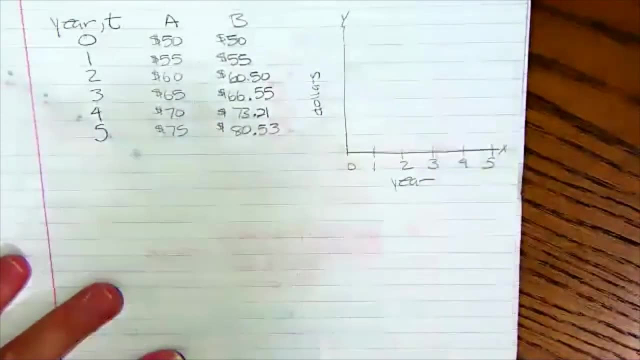 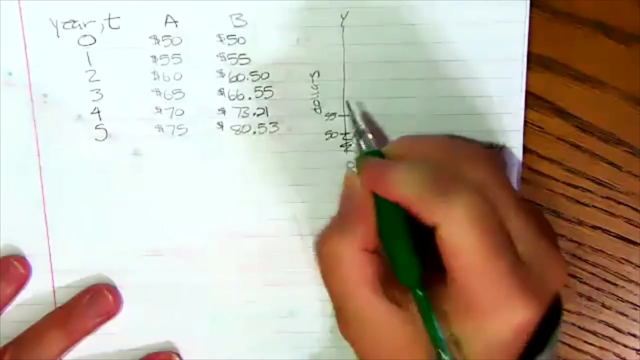 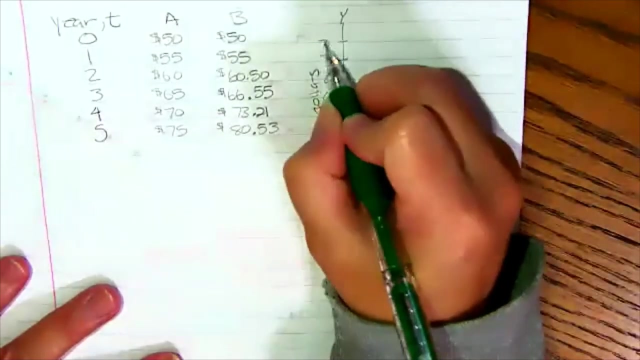 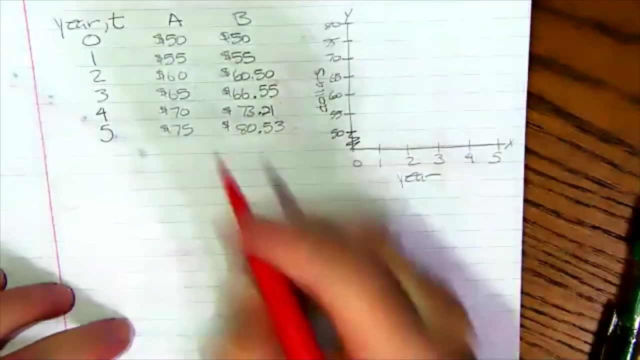 My y-axis will be the dollars And my y-axis is the year. So I've got $1.. And let's go with 50, 55,, 60,, 65,, 70,, 75, 80.. So let's graph these guys. 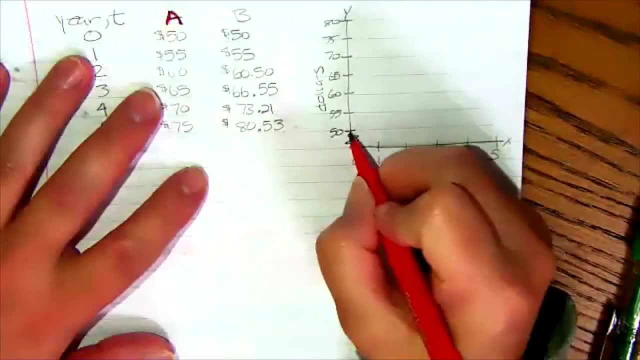 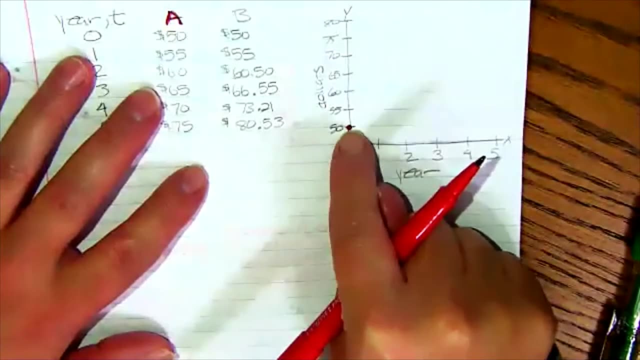 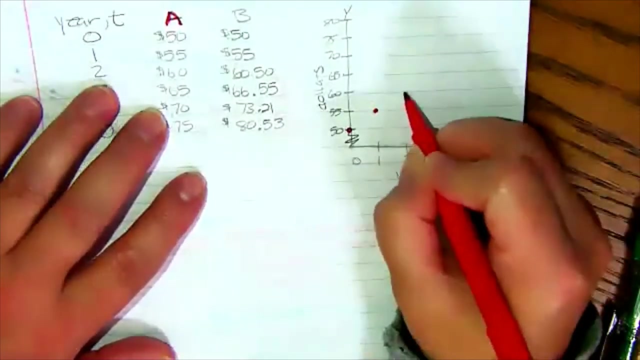 So account, A simple interest: After one year We start with $50.. So at zero years we're starting with $50.. After one year we've got $55.. After two years we've got $60.. After three years we've got $65.. 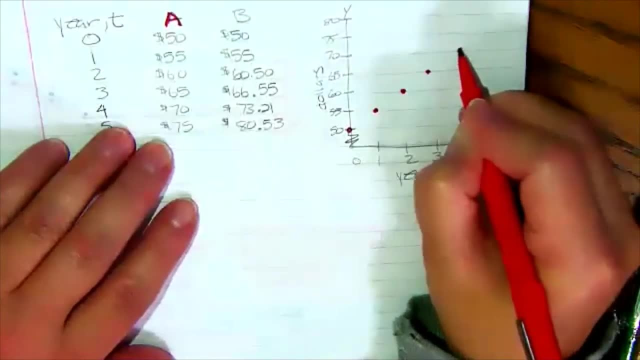 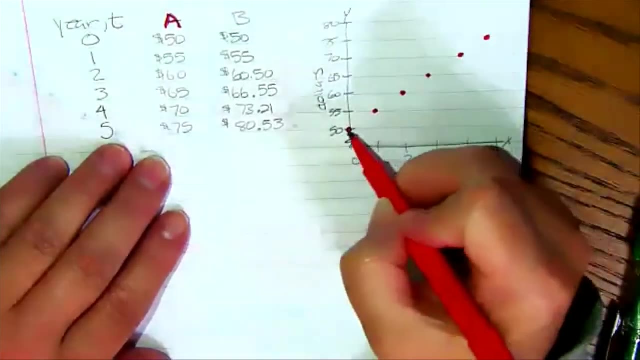 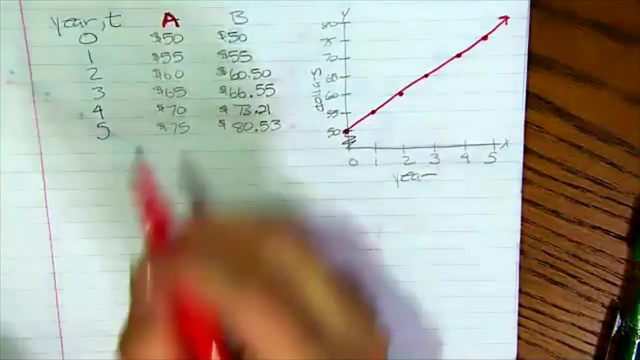 After four years we've got $70.. And after five years we've got $75.. When I look at this, it looks like it's a pretty straight line. So let's take a look at our table just to confirm our rate of change. 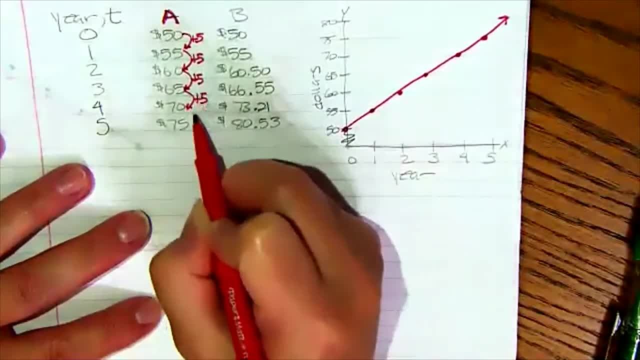 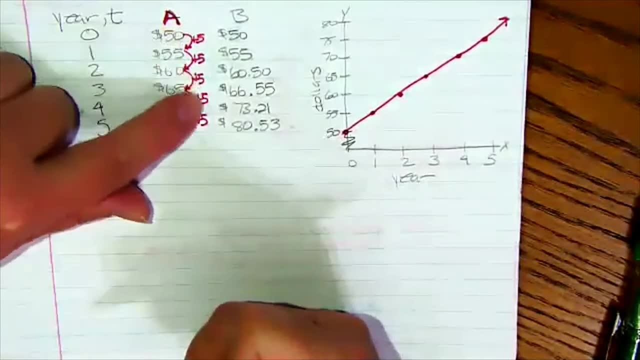 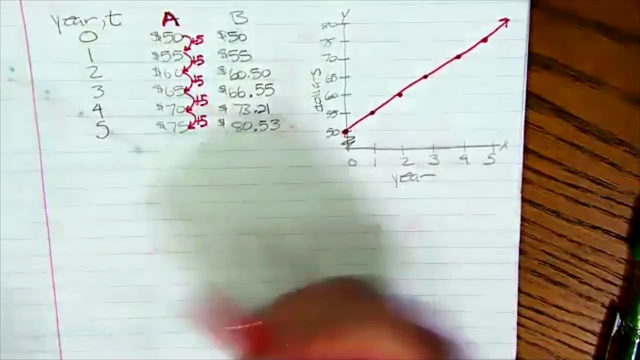 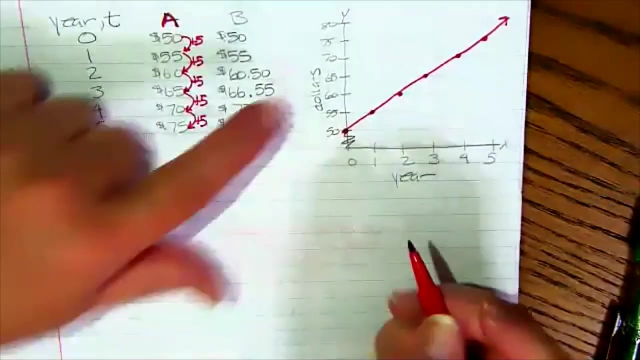 Oh, look at that. We have a constant rate of change. It increases by five every year. It only increases by $5 every year. That's the same. That is constant. So what can we say about graph A? It is positive, or the amount increases. 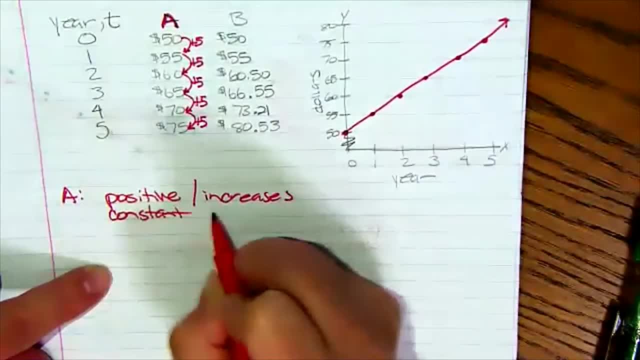 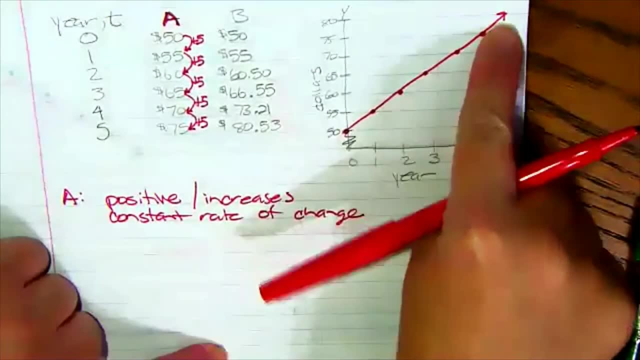 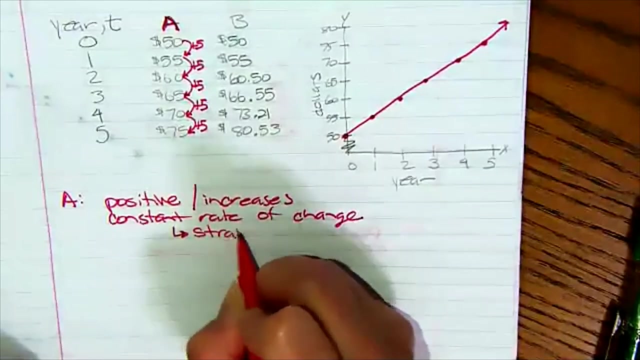 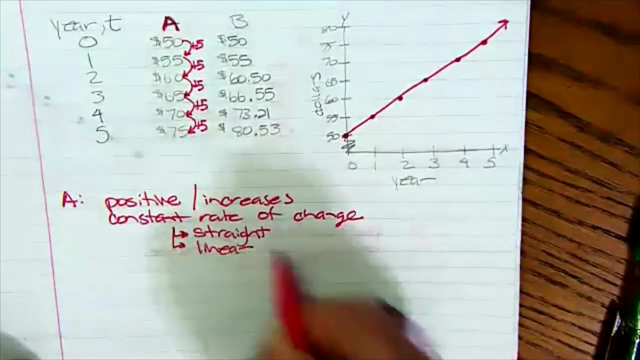 We have a constant rate of change, proven right here. I mean, this looks like it's a straight line, but we just proved it with the table, So that means our line is straight, Our graph is straight, which means we have a linear function. Now let's graph the second account, account B, compound interest. So we're starting with $50. And after one year we have $55, just like account A. But now, after two years, we've got $6.50.. Not that big of a deal. 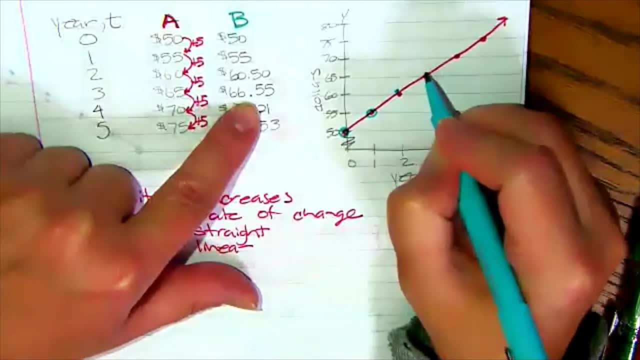 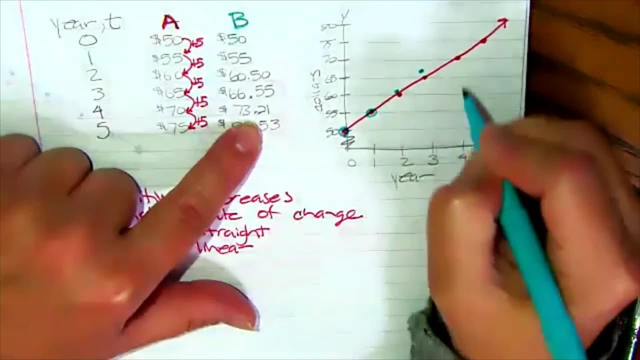 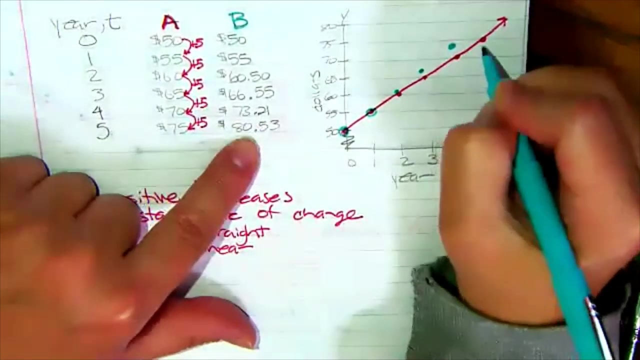 After three years we've got $60.. After four years we've got $76.55.. After four years we've got $73.21.. And after five years we have more than $80.. So to look at this, 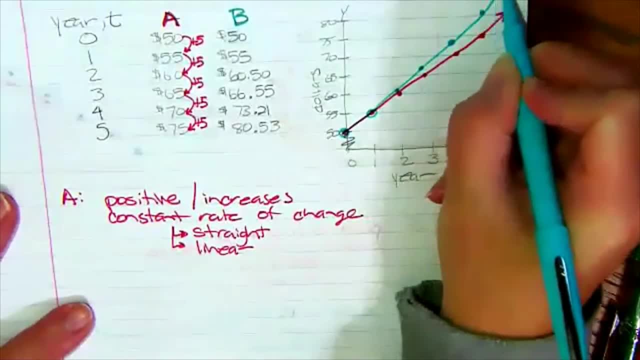 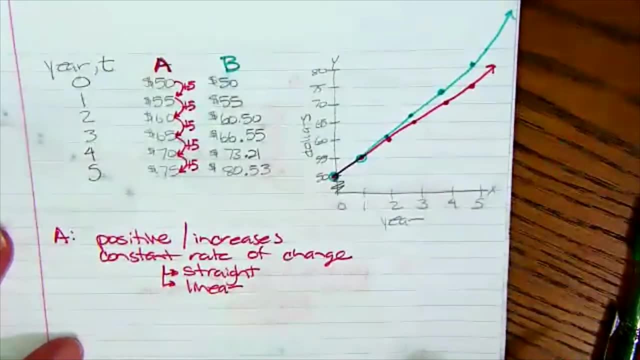 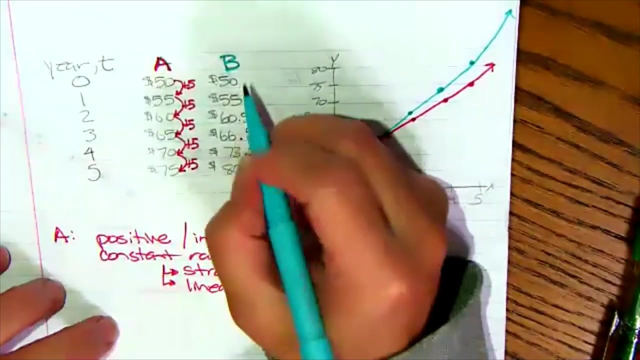 shh, It is a curved graph. It doesn't look linear, It doesn't look like a straight line, It's curved. But I want to be sure, so I'm gonna check my rate of change. So here I have plus five. 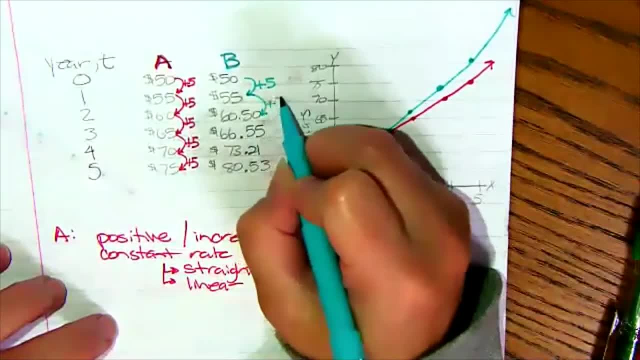 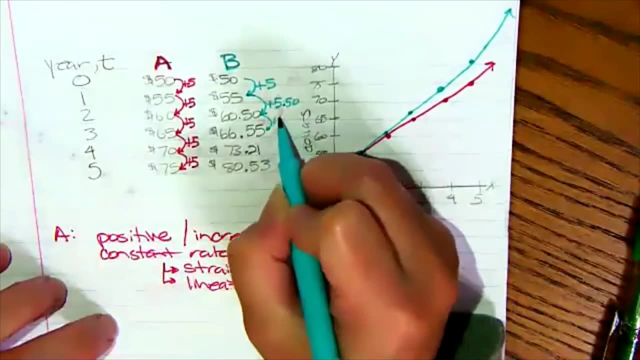 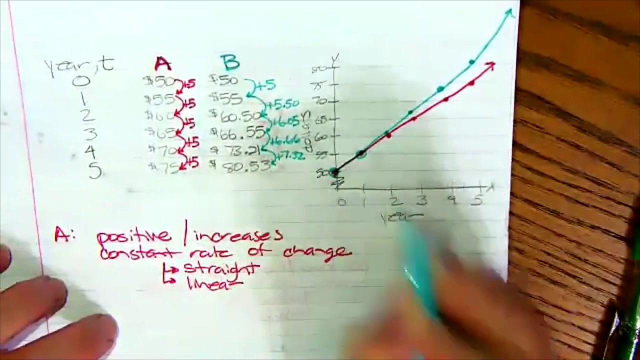 Oh, Right, here plus five dollars and 50 cents shh, plus $6.05.. I can see that my rate of change is not constant. My rate of change is changing. It's not the same, It's not constant. 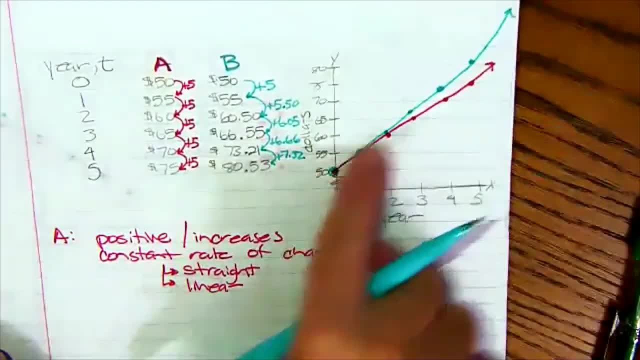 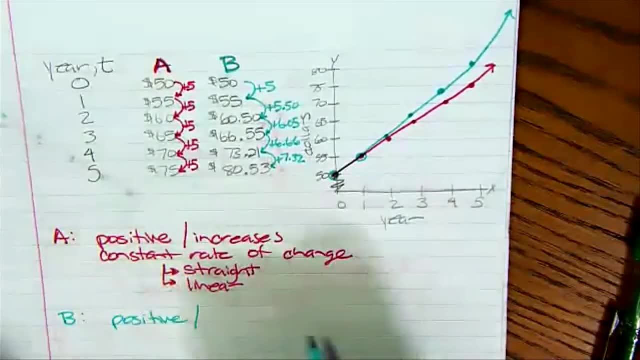 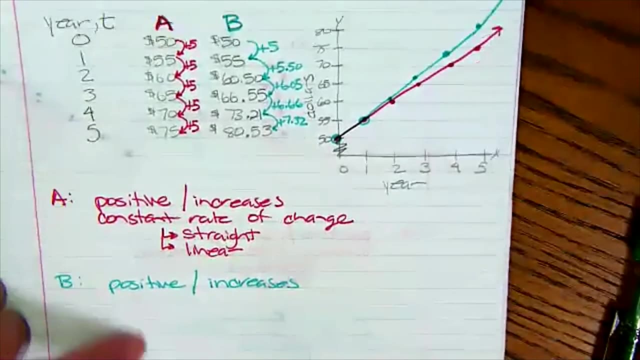 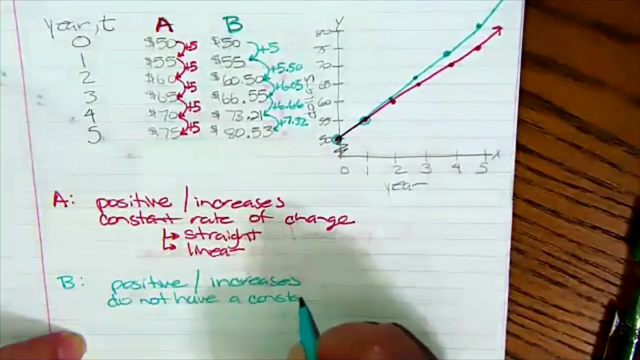 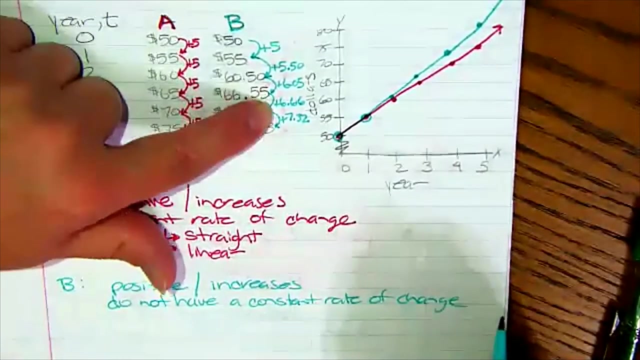 So that confirms that this is not a straight line. It's curved. So what can we say about account B? It's still positive, The amounts are still increasing, But I do not have a constant rate of change proven by the table, which means my graph is curved, which means